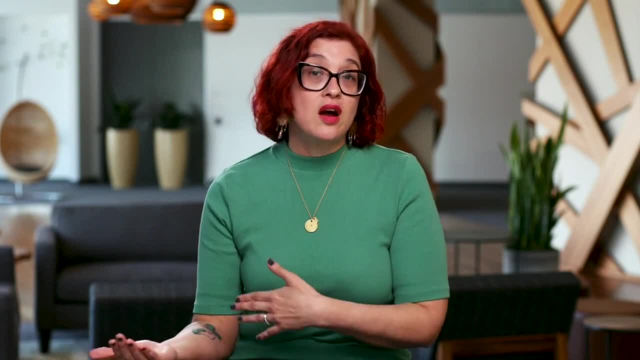 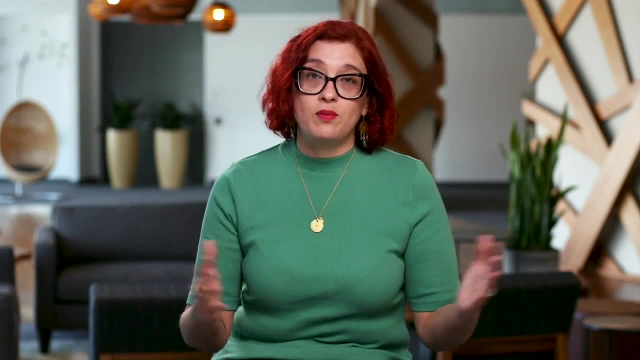 get your product to the right influencer and they organically start talking about you, then that can help you create a lot of buzz and generate awareness to a new audience that you wouldn't have been able to reach otherwise. So, Google Developer Studio: part of what we do is bring a community of developers together. 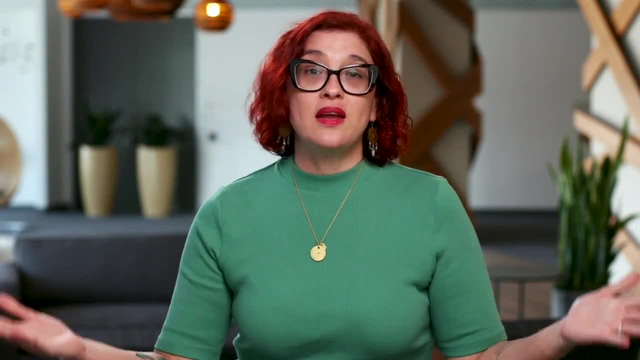 at events, And part of my job is to reach as many of those relevant developers and let them know that they're making a difference and that they're getting their work done. My job is to be able to show them content that they want and show them that they're. 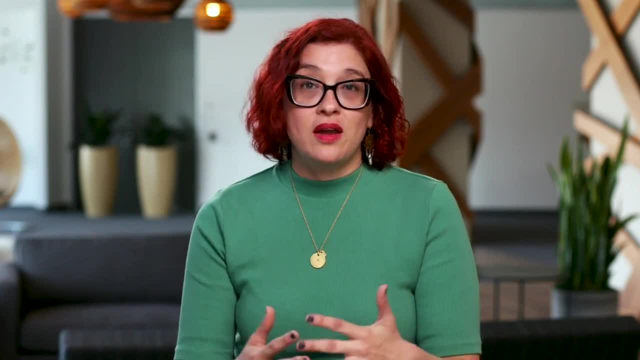 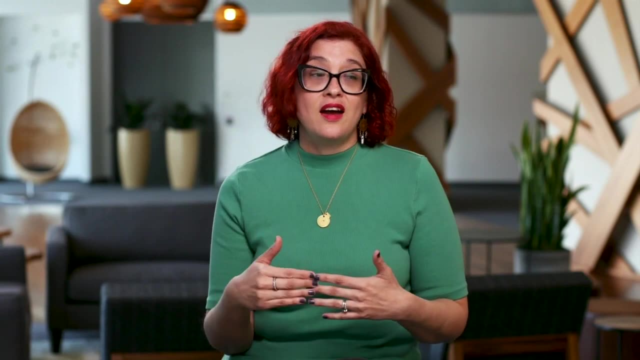 making a difference and to show them that they're making a difference and to show them that they're about the event and the announcements coming from that event. so, as the developers are watching our content and having conversations about what they're seeing, then that's exactly what we want, right? this is what we talked about is. 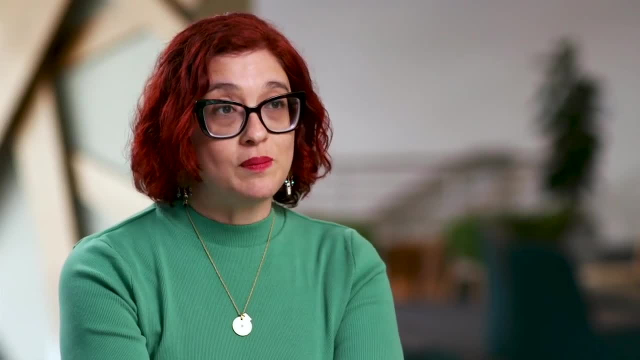 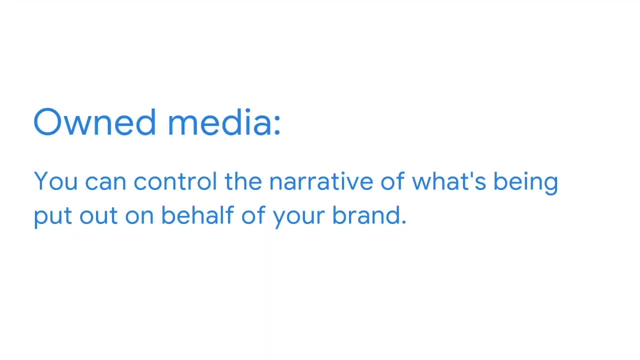 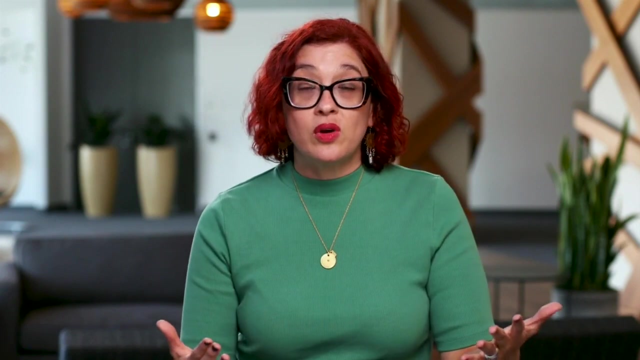 that natural buzz that's coming up with owned media. since you own the channels, you really have the benefit of being as creative as you possibly can get, and you can control the narrative of what's being put out on behalf of your brand, whether that's your personal brand or the business that you're running. you can. 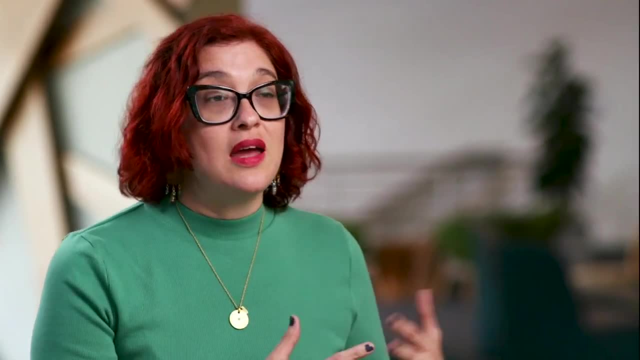 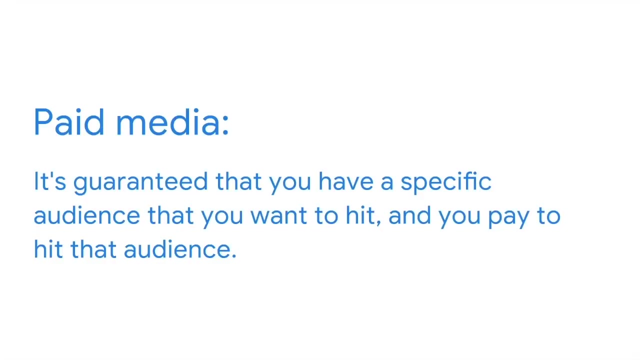 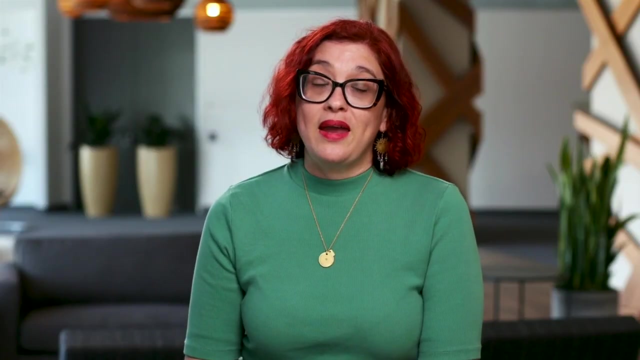 own your Twitter, your Facebook, your Instagram, your social channels. these are all different distribution networks that you own and control what goes out on them. with paid media, it's guaranteed that you have a specific audience that you want to hit and you pay to hit that audience. the great thing about paid: 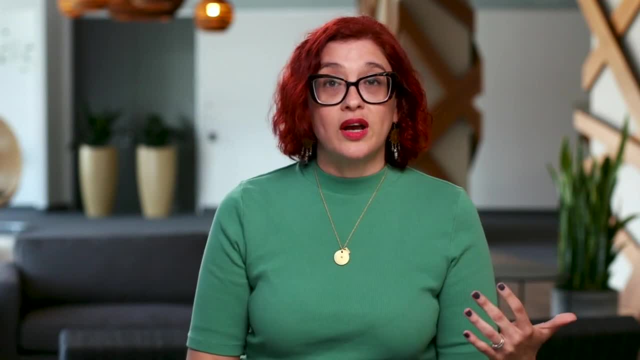 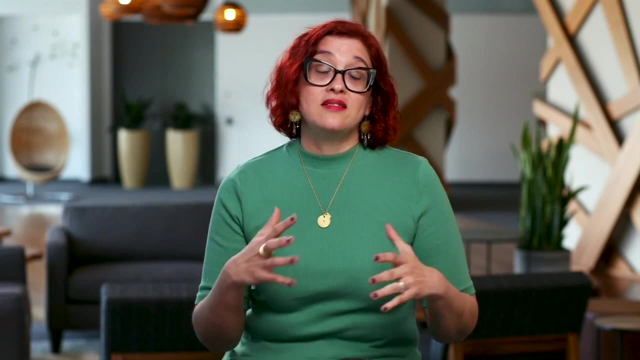 media is with social networks like Facebook or Instagram, especially for a local business. a small budget can actually make a difference in your business and you can make a difference in your item fascination. it can also help make quite a big impact, and some of the things that we can do with organic media- owns media- is test out the best kind of 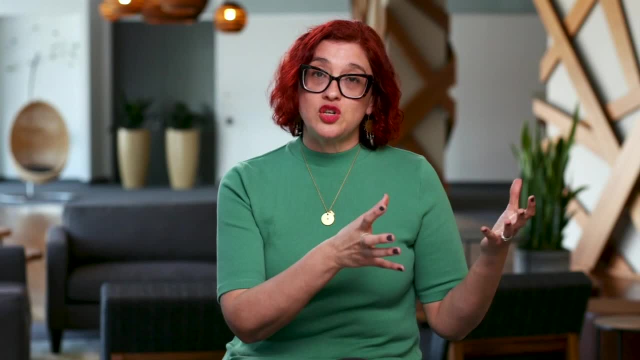 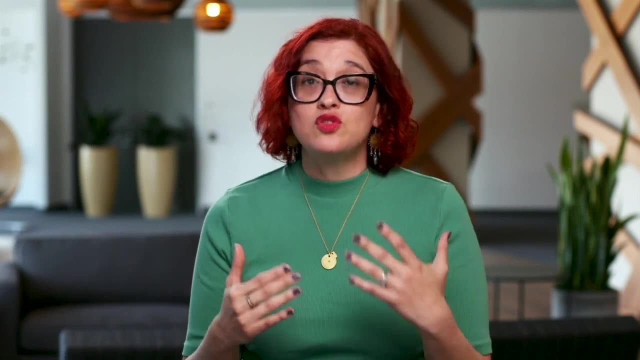 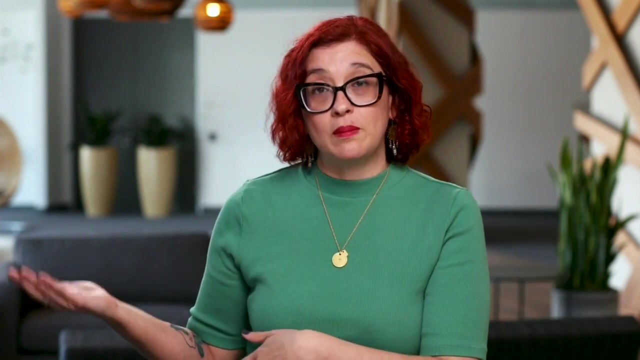 messaging and creative assets, and when something is starting to percolate and gain traction, we can use paid media to boost that content, and that's really a huge advantage to how you can use your owns channels and make smart decisions about where to put your money using paid. there are so many different social 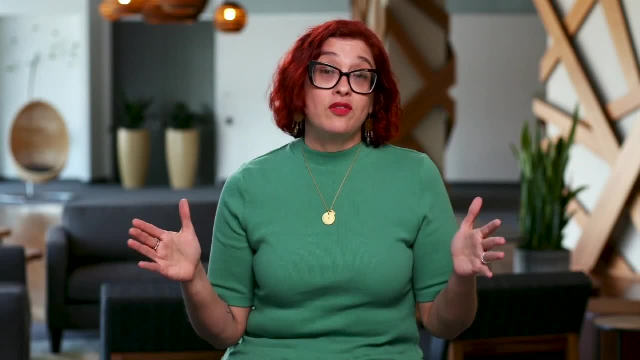 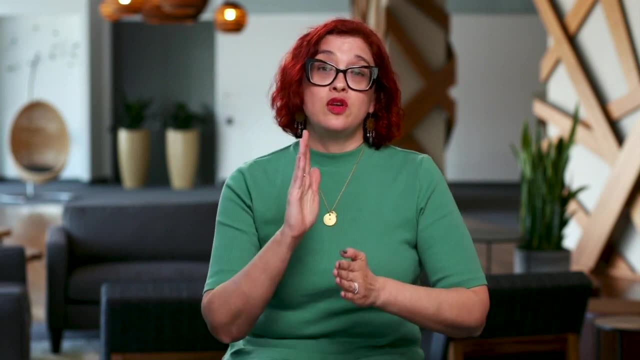 and they each offer different benefits. However, once you've really found your niche and you know where your audience is and you're really owning that channel, the mix of using earned, owned and paid on that one channel is going to get you much, much further.